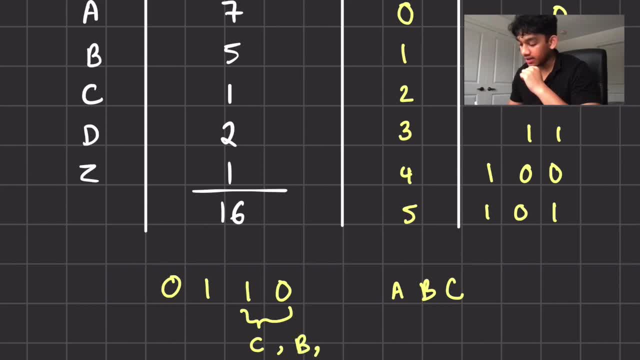 Also being just B A right, So we can actually have A B, B, A, ABBA, And we don't want that. We don't want any ambiguity when we're working with this right. So what we do to avoid that? 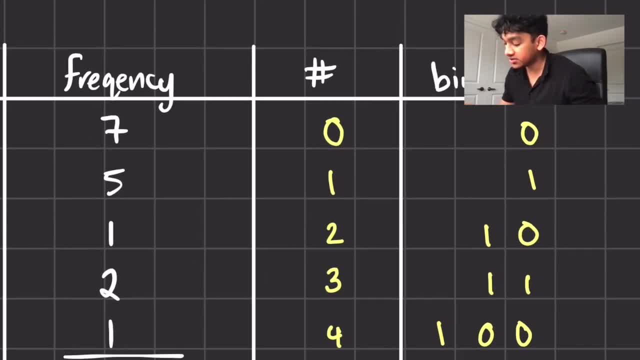 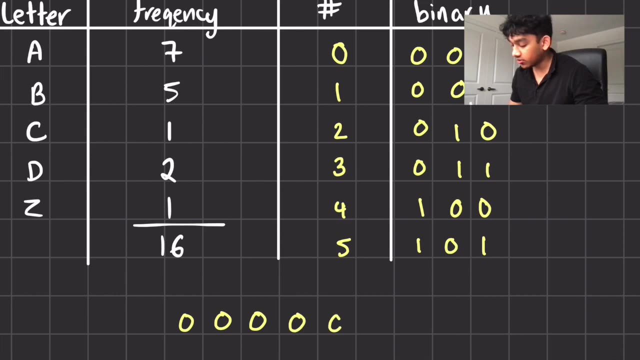 is, we make sure to have the rest of the bit. So if it's zero, we're going to have three digits here. So three bits actually: Zero, zero, one, zero and zero. And now you're going to use this: So zero, zero, zero, zero, zero one. You're going to notice that they're 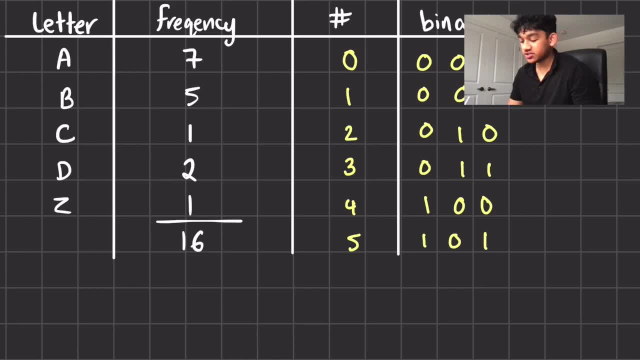 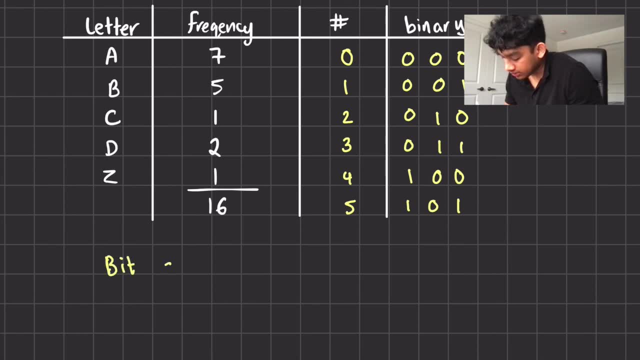 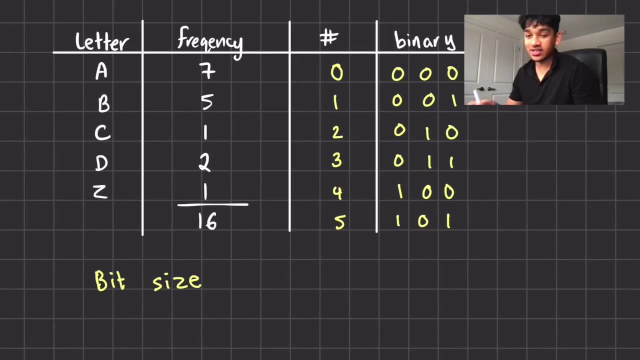 separated by three bits. Now the issue is that even though it's small, it's still not optimal. We can actually see the bit size here by calculating it. So we know that A takes three bits. B, C, D, Z- they all take three bits each. There's seven A's, and each A takes three bits. 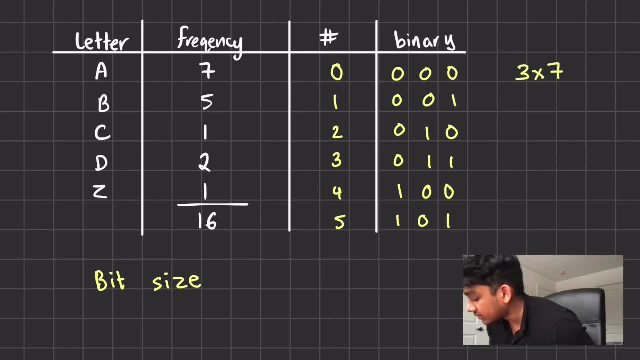 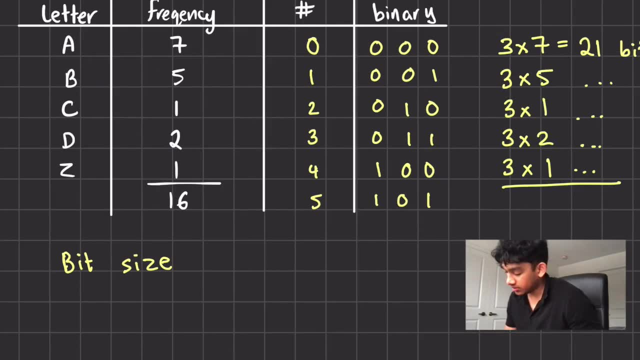 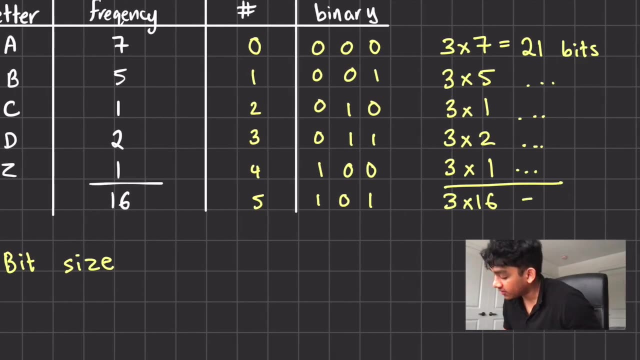 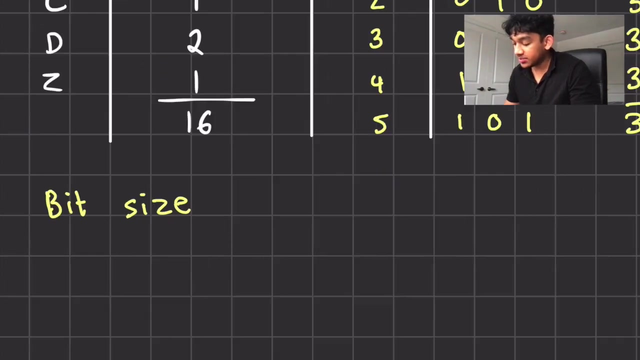 so that we know: Three times seven is 21 bits. You can also just do three times 16, because we know that there's 16 characters and each one takes three bits, which is just 48 bits. So the way you know how many bits you need is: it's basically going to be two to the power N of something. 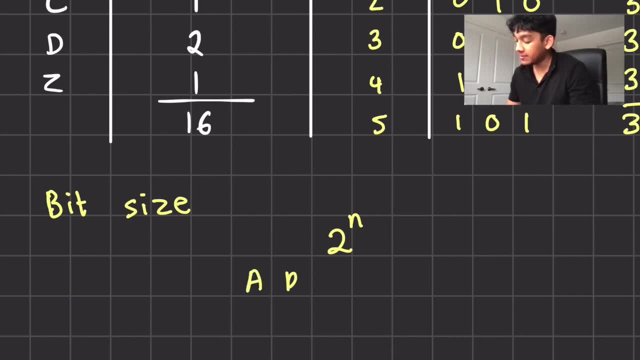 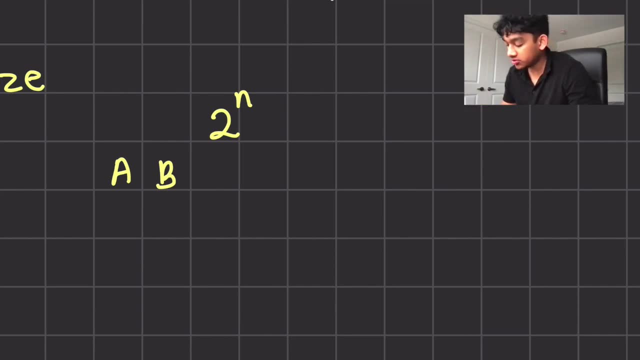 For example, if you have two characters, let's say A and B, And we need to write it in a way, using bits, We count how many items we have. So we have two characters here and we need to find a number to the power of two that will suffice us. So in this, 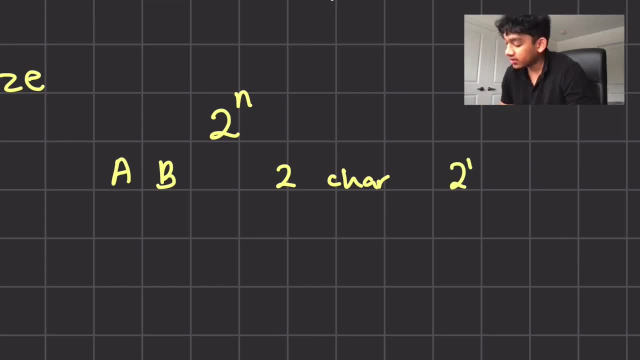 case it would just be two due to the power one. So that means we only need one bit, because the power tells us how many bits we need. So if we have one bit, that means it could be either zero or one, And we can write: A is equal to zero, B is equal to one and we're done. But let's say we. 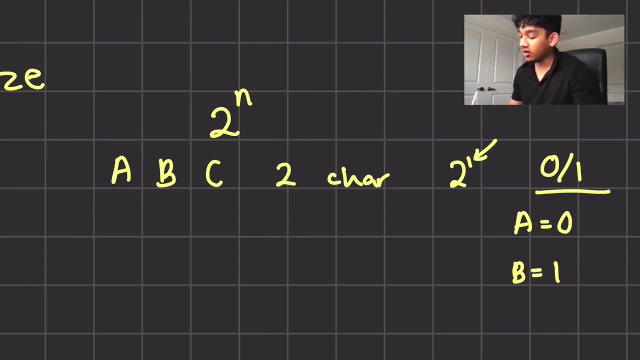 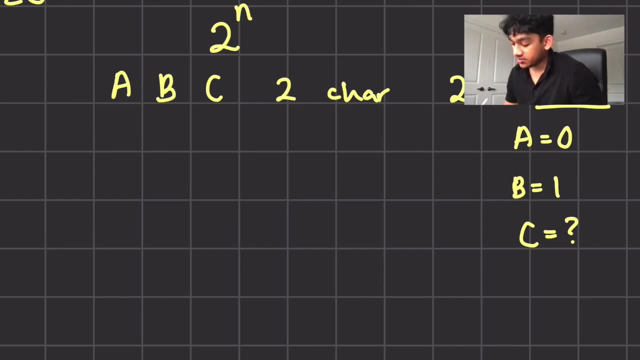 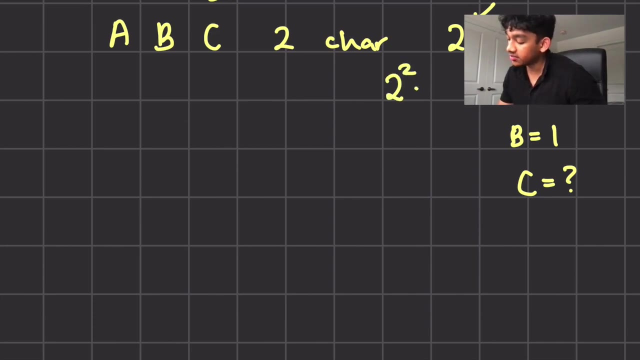 add a third character, let's say c, right. all of a sudden, what could c equal with one bit? because we already took zero, we already took one. there's no way of doing it. so what we do is we use the next power to two right. so two to the power. two is going to be four right, and we can see this by: 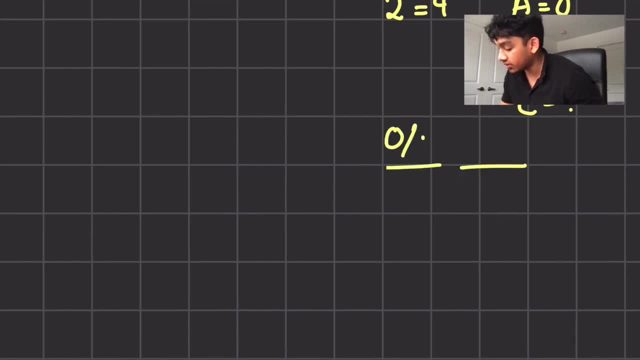 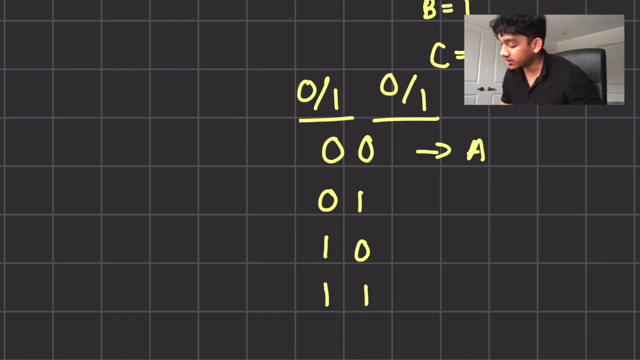 having two bits right here, so zero and one, zero and one, and we're going to have four different combinations. now we're going to have zero, zero, zero, one, one, zero, one, one right, and even though we don't need four, we always go up right. so this can be a, this can be b, this can be c, and if we 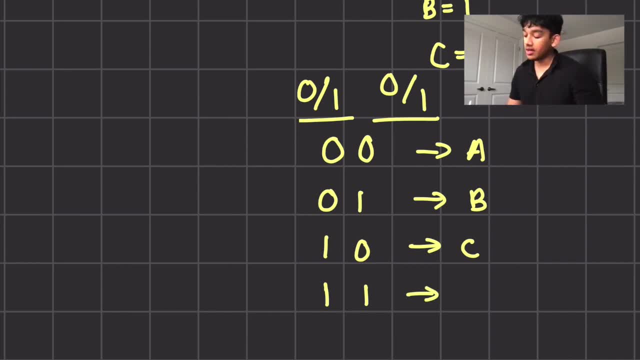 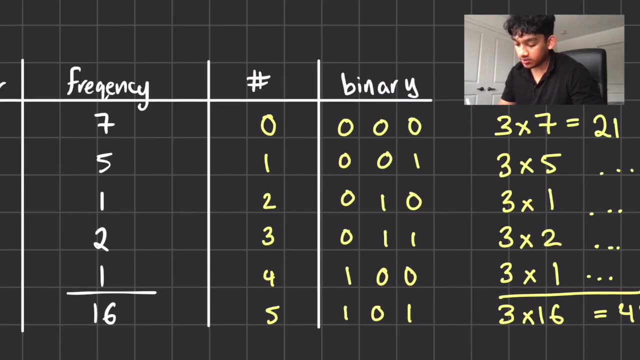 have another value that we never need. it could be one one, right? uh, basically, what we want to do is just find two to the power something. so in this case, we have one, two, three, four, five. we have five different things, so we're gonna have to do two to the power three. 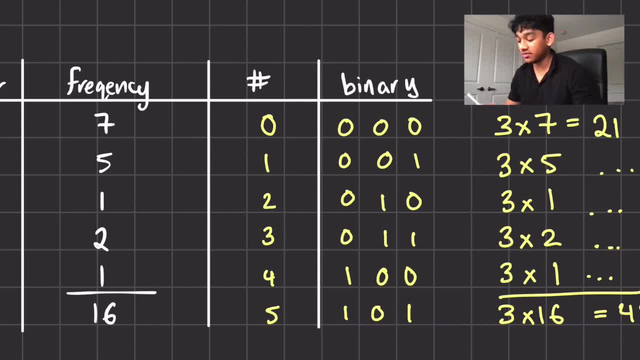 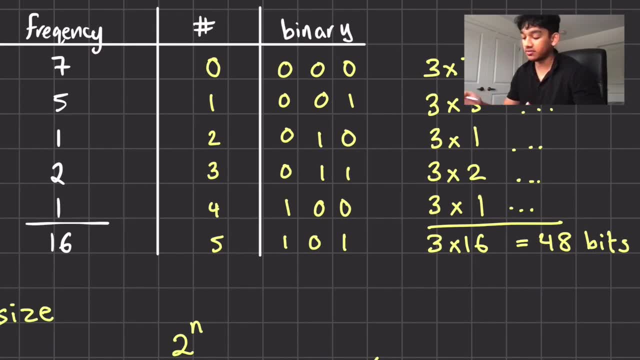 you is eight, because two to the power two is four, and it's not enough. that's why we need three bits here. so even though we don't use every single combination of bits, we we still have enough to make it work. okay, so what i've done here is i just made a set with all the characters and their 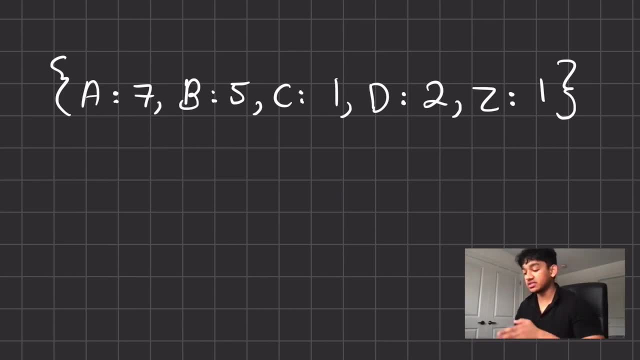 frequencies right beside them, colon separated right, so we know that a has seven, b has five, and so on and so on. so this is how the hoffman algorithm works. first we take the two smallest frequencies, so in this case we're gonna have z and we're also gonna be using c and what we're. 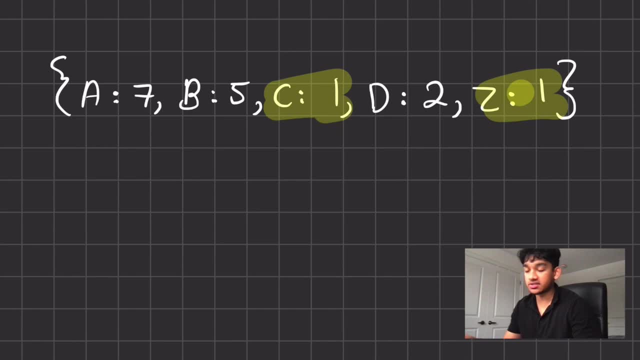 gonna do is make a binary tree where c and z are siblings. so we're gonna have c one here, we're gonna have z one here, and we're gonna come, we're gonna add these up to a single node and the node is gonna have the sum of the two frequencies, which is two. 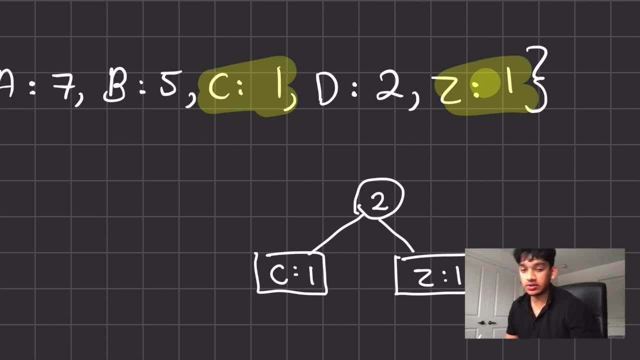 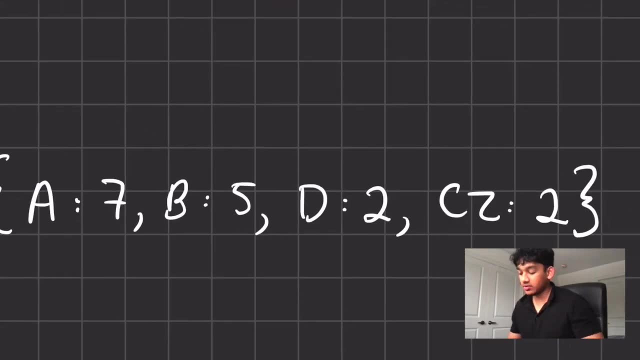 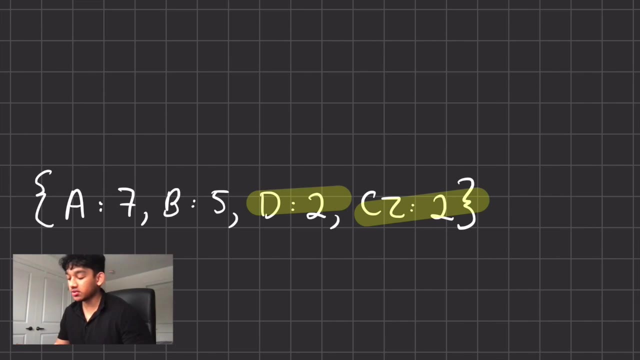 now, all of a sudden, we have a new element in the set, which is two right, and we can represent that as said, cz. so now we have a7, b5, d2, cz2, d and cz are the smallest values in this case, because this has a frequency of two, so that has a frequency of two. so what we're going to do is we're going to 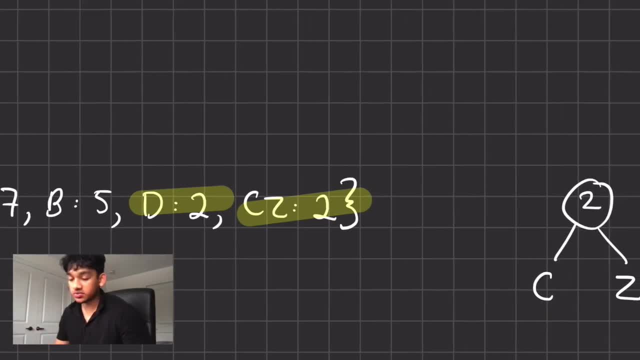 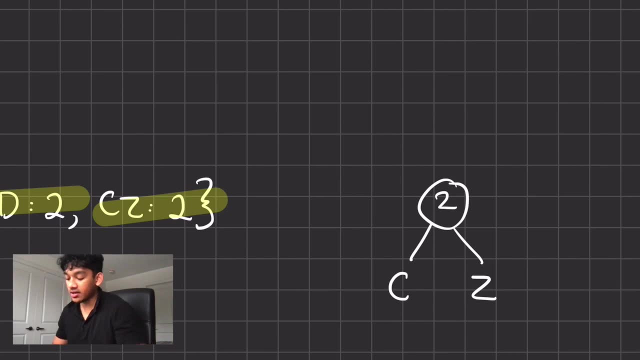 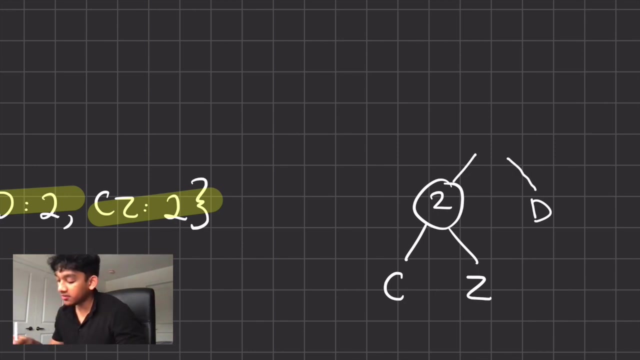 join these and they're going to be siblings now. so these are going to be siblings with said z. it's going to be the. it's going to be siblings with the node. that's apparent for both of these nodes. so d we can actually just write here. d would be here, and now we're going to have the sum of these two. 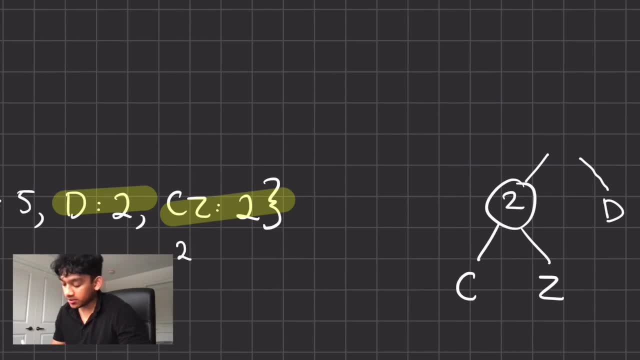 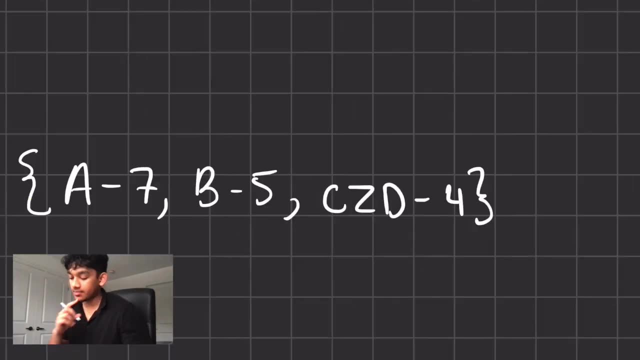 frequencies. so said z is 2, d is 2, 2 plus 2 is equal to 4.. so we have 4 all the way up here and this is going to be our tree for now. so we know that b and c is at. d are the smallest values. 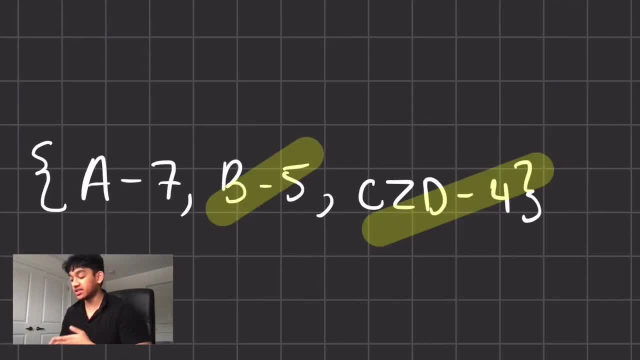 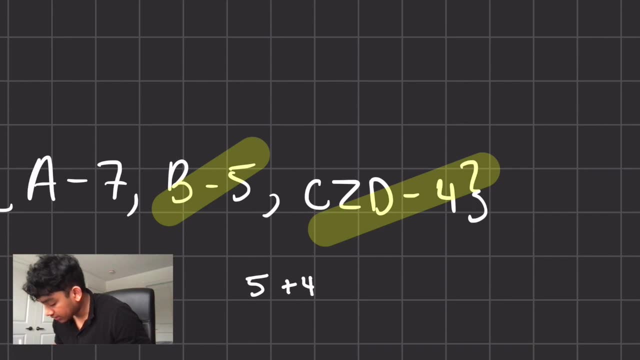 now, and by the algorithm this means that b is going to be siblings with c, z, d, so the parent node is going to be the sum of these two, so we know that it's going to be five plus four. plus four is equal to nine, so all we do now is 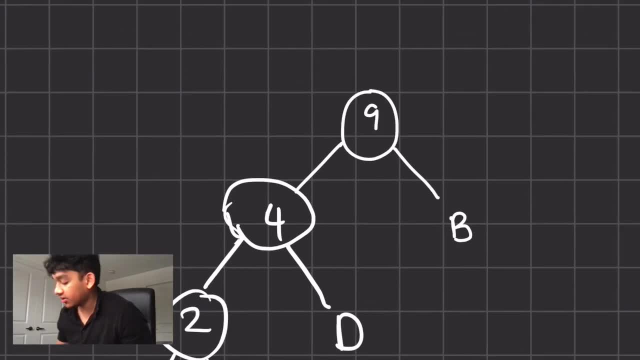 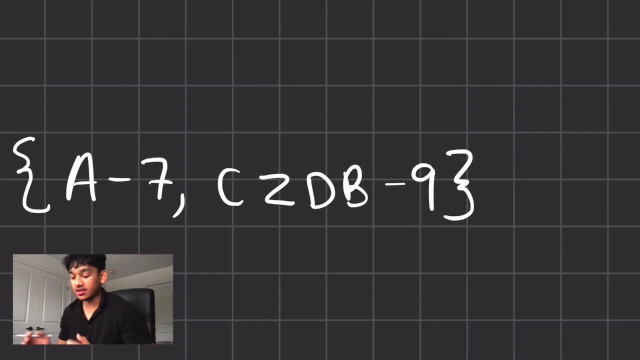 make space for b and we put the sum of nine on top and this is the final set. we only have two values left, so they're obviously going to be the smallest ones and we add the two, so a is going to be siblings with this node right here, the nine. so this is a tree, what we're gonna do. 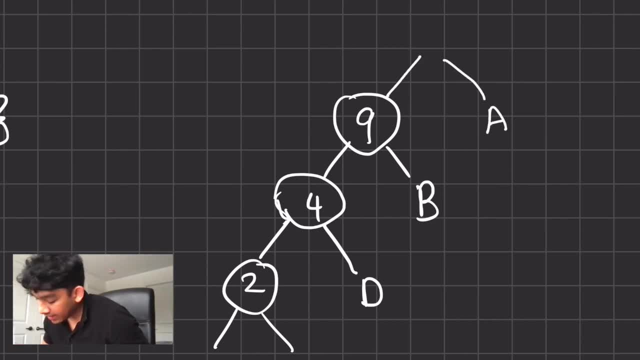 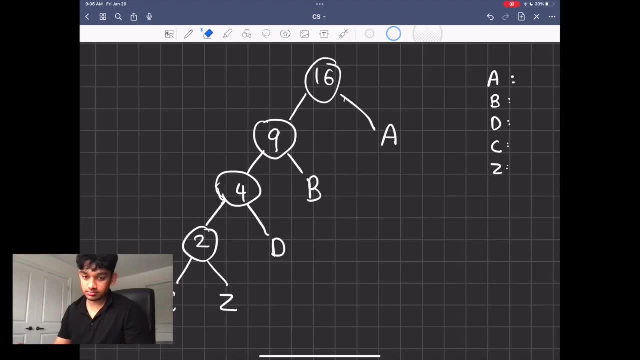 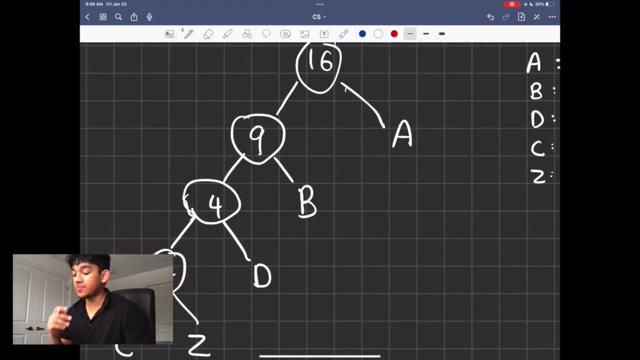 is put a here and we're gonna add the sum again, so it's gonna be seven plus nine is equal to six and 16, and 16 is going to be at the top here. so we finally constructed this tree and we call this tree the hoffman tree, and what we're going to do next is we're going to lift, we're going to label. 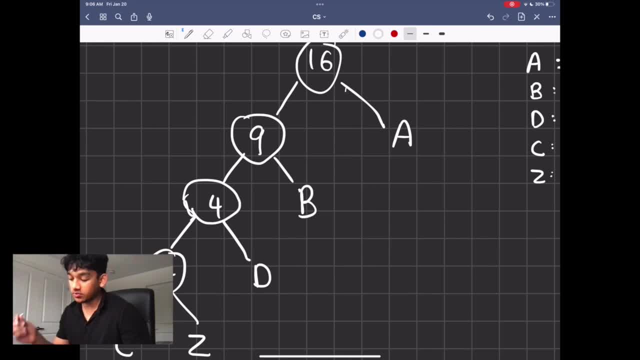 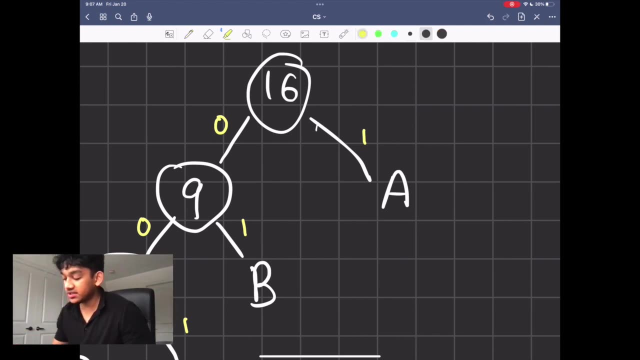 every single left branch as a zero and the right ones as a one. zero, zero, zero, zero, one, one, one one. and we're going to get each. we're going to label each code as a path to get there from the root right. so from, if you want to go from 16 to a, you're going to go one. 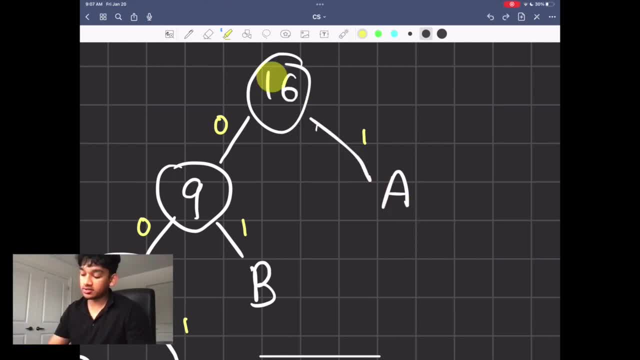 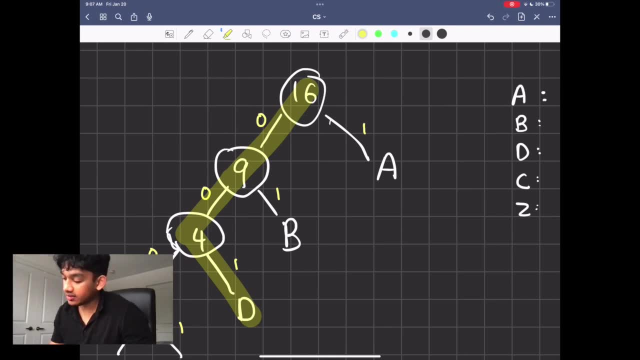 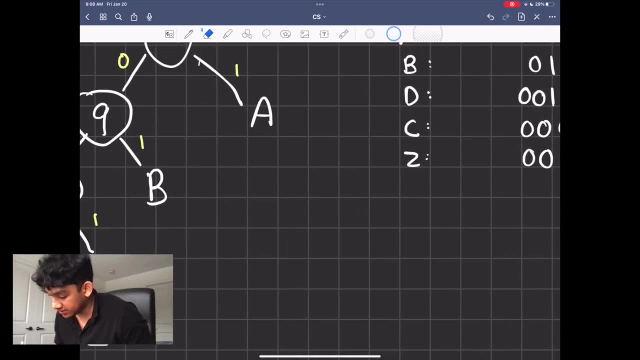 if you want to go from 16 to b, you're going to go zero one. for d, it's going to be zero, zero one, and so you get. if you repeat these steps for every single one, you're gonna have this legend right here. if we actually try to write the sequence a, b, c like we did before, we're gonna write: 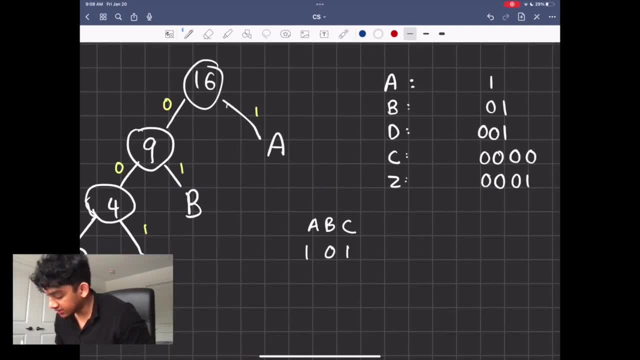 one, zero one, and then c is zero, zero, zero, zero. so one off the top. we'd only know that one character starts with one which is going to be a, so we know that that's going to be a zero one. so there's no zero in the sequence right, there's only zero one. so we take that and we.